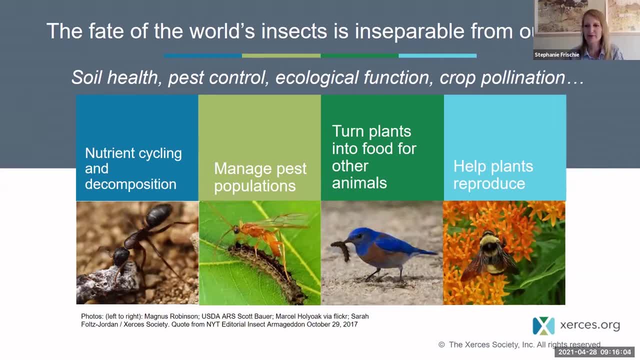 insects is inseparable from our own. Insects perform all these types of functions. They're important for soil health, pest control, other ecological services, including crop pollination. So, as are shown here in these photos, insects are important for their role in nutrient cycling and 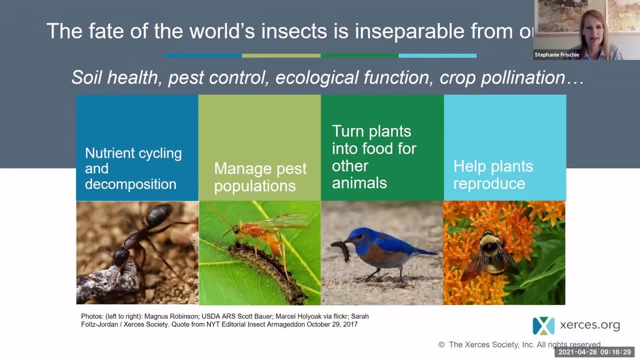 decomposition. We'll be talking more about those insect groups today, Also for how they balance or manage pest populations. Insects also turn plants into food for other animals, And you know the way that birds really rely on caterpillars to feed their young chicks is one example of that. 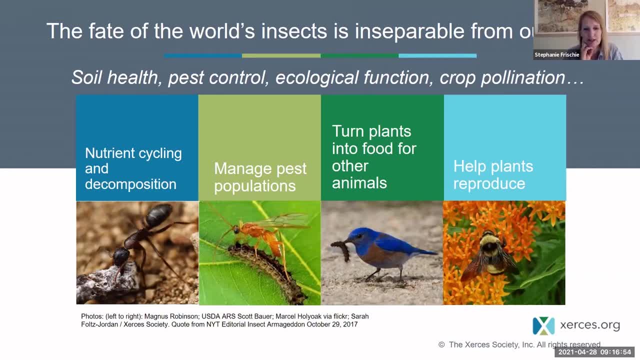 And then for us, many of the fruits and vegetables that we eat depend on insects for their pollination. So again, those insects are turning plants into food for us as well, And then they also are important in their role in helping plants. 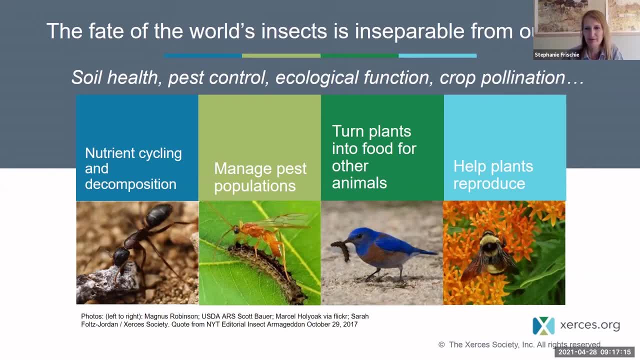 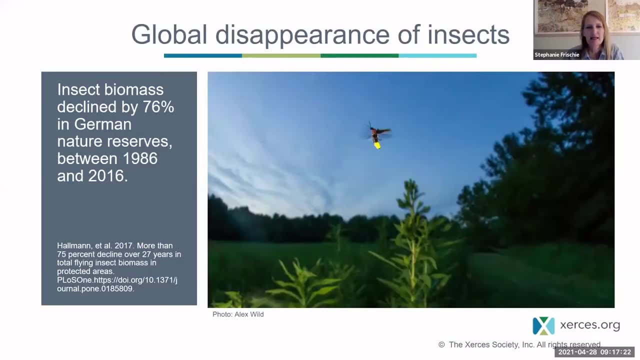 reproduce and sustain those plant populations. Yet so many of the invertebrate and insect species that we eat, they're not all the same. Insect groups are in decline. Decline means that the number of individuals or the number of species are decreasing. In a telling study published in 2017, the biomass of insects in nature reserves. 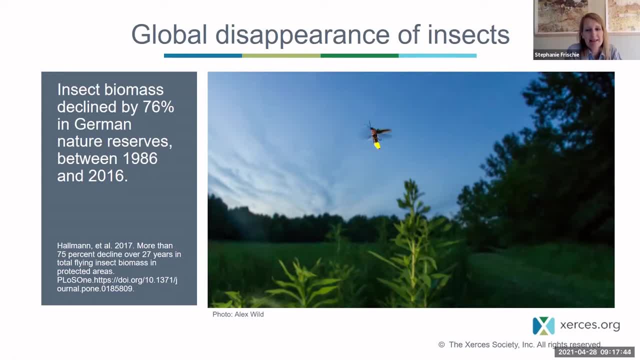 in Germany decreased by 70%, And this is in nature reserves, where presumably insects would be the most protected from various threats. But despite that, such significant declines were measured. I imagine most of you can recognize the insect in this photo. It's a firefly, or also known as a lightning bug. 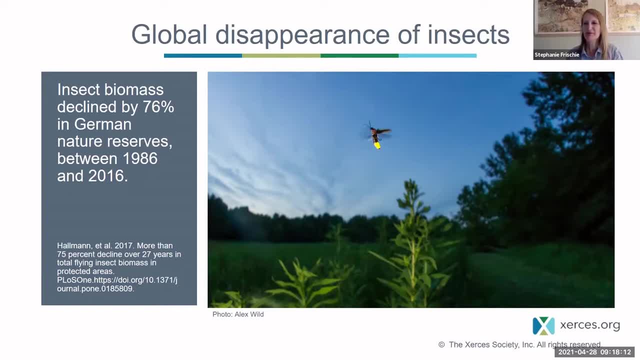 It's fairly recognizable by most people, And I'm wondering though: did you know that fireflies are actually soil invertebrates? If you didn't know that already, you'll be learning more about that soon too. If you didn't know that already, you'll be learning more about that soon too. 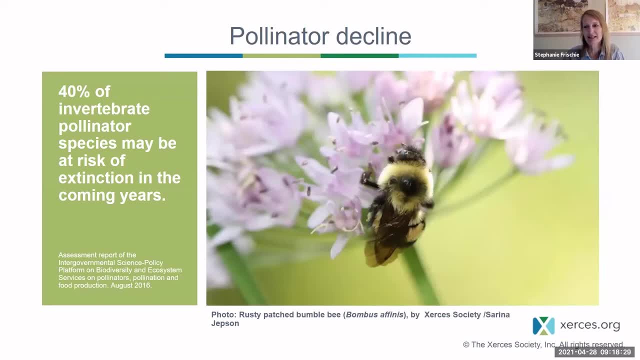 иейル that are in decline By by one estimate of a global intergovernmental report: 40% of invertebrate. Además, 40% deiers de harboras. humanity a posse- intergovernmental report. 40% de quierar, a posse in Mythical service in China, at risk of extinction. 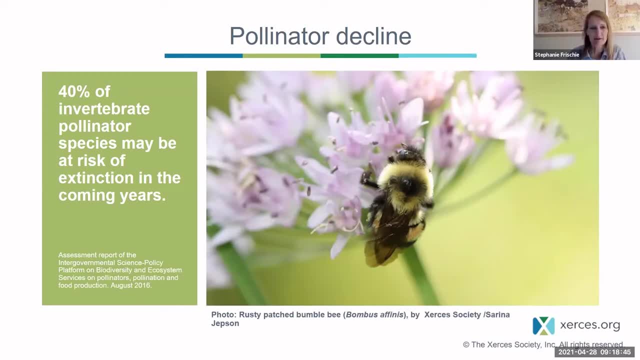 I think the media and the news have covered. I think the media and the news have covered the difficulties facing facing honeybee populations pretty well, But honeybees are actually only one type of bee and they were brought to the U? S. 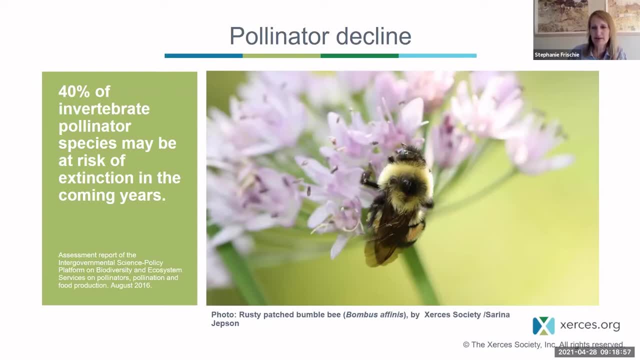 But honeybees are actually only one type of bee and they were brought to the U? S to the US centuries ago from Europe. They're considered a managed species and they're non-native. However, in North America there are nearly 4,000 other species of wild native bees. 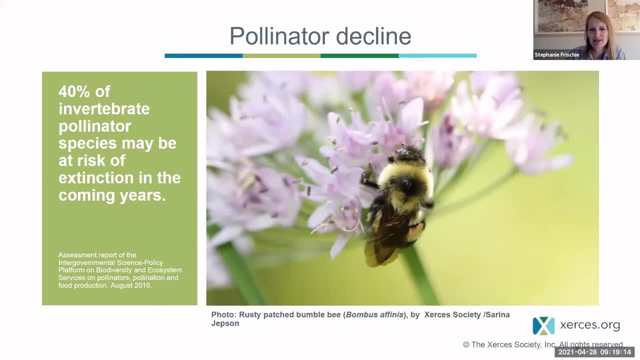 and this photo shows one of them. This is the rusty patched bumblebee, so a midwestern and formerly eastern species which was added to the federal endangered species list in 2017.. This is the first bumblebee to receive, or actually to need and receive- this kind of protection. 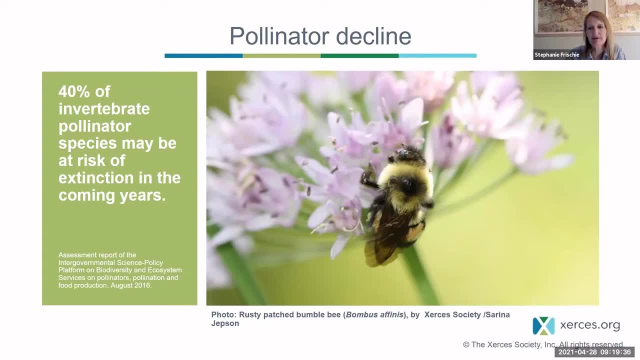 However, overall, relative to other species groups, very few bees, butterflies and other invertebrates are on the endangered species list. This doesn't mean that they're safer from extinction. it really points to how little attention has been paid to these species and their distribution to date. 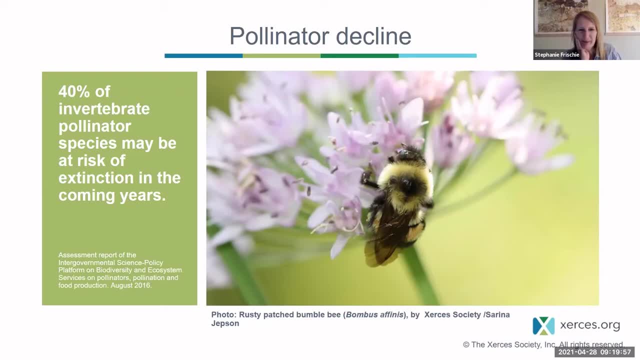 All right. another little question here is: is a bumblebee a soil invertebrate? What do you guys think? Okay, I hope this isn't a spoiler, but the answer is yes, Bumblebees can be considered soil invertebrates, in addition to being considered pollinators. 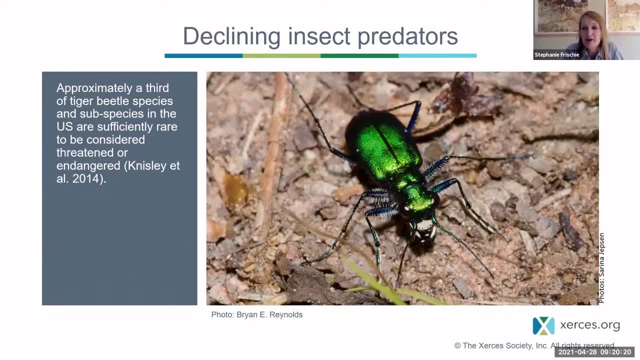 So not only bees and butterflies, but also predators or natural enemies, such as this tiger beetle, which is a species of the eastern US pictured here. Decline has also been measured in these predatory groups- Approximately a third of tiger beetle species and subspecies in 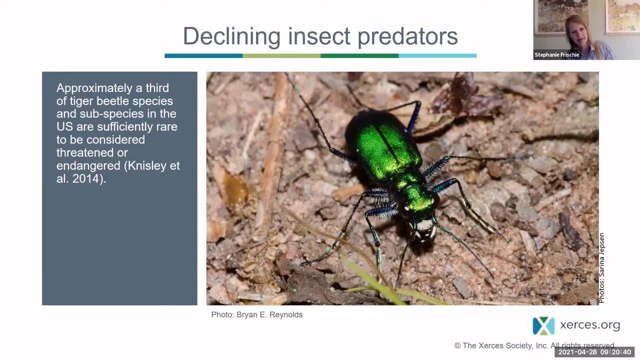 the US are sufficiently rare to be considered threatened or endangered. So, okay, perhaps the fact that this beetle is pictured on a background or on the soil surface it gives us a clue that tiger beetles- yes, these are also soil invertebrates. 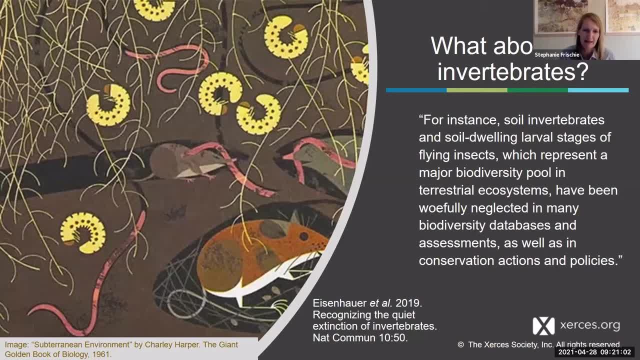 So, almost anywhere that invertebrates have been studied, what's been measured is that they are in decline. But what about soil invertebrates? Well, actually, our scientific and ecological understanding of soil invertebrates is still at a fairly basic level. This quote is from a recent review that looked at trends in invertebrates. 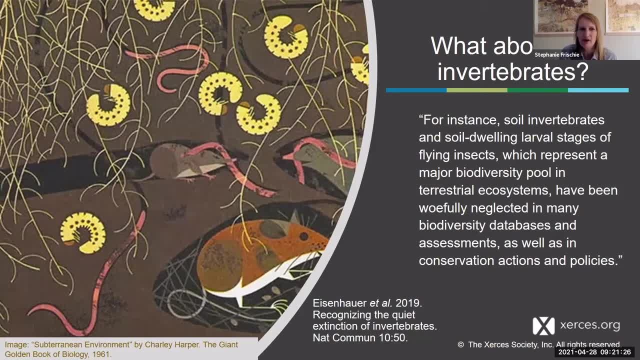 And the authors said that, for instance, soil invertebrates and soil-dwelling larval stages of flying insects, which represent a major biodiversity pool in terrestrial ecosystems, these groups have been woefully neglected in many biodiversity databases and assessments, as well as in conservation actions and policies. So they're basically saying: 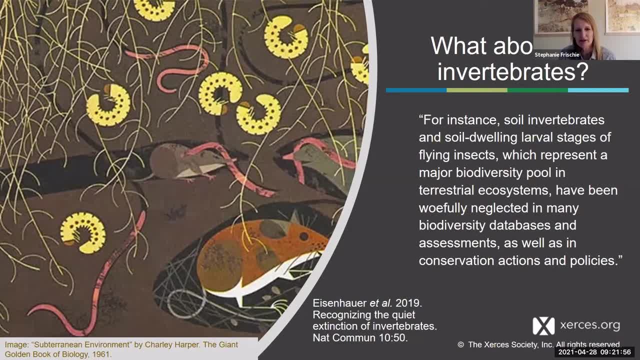 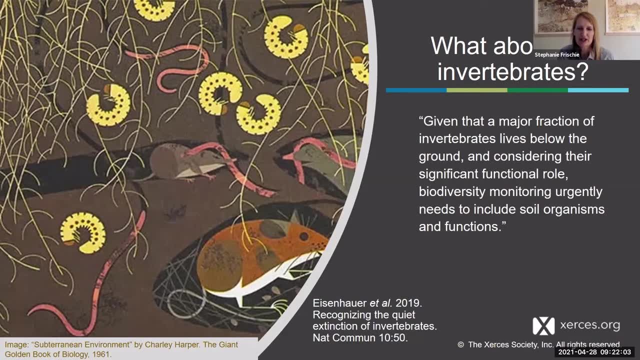 these are such important groups ecologically that they've been understudied so far, And so their recommendation is. given that a major fraction of invertebrates live below the ground, and considering their significant functional role, biodiversity monitoring urgently needs to include soil organisms and functions, And there are certainly research groups that do study soil. 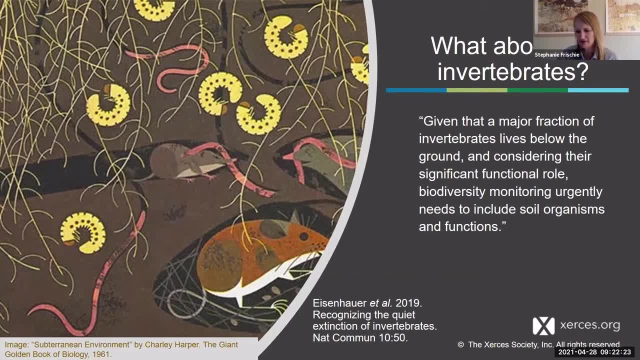 invertebrates, but compared to us, not other insect and invertebrate research, less is still known about those groups, So it's hard to measure what the decline is, if such, or what the status is of a lot of these groups. 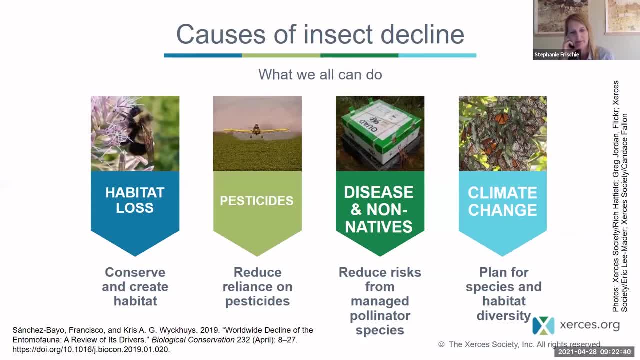 since so little is currently known. This slide shows some of the four primary causes or categories of insect decline. So again, in almost every location or situation where they've been studied, insects are in decline, and these are the major causes for that. 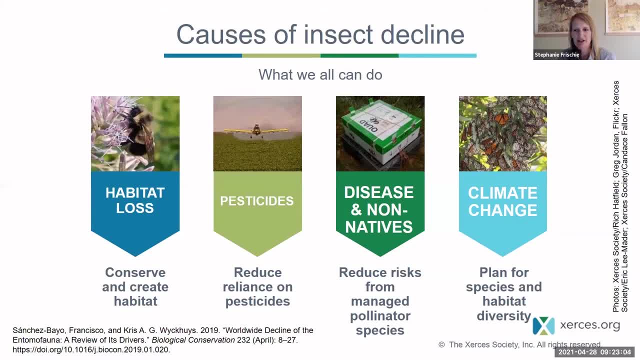 And then, at the bottom of the arrows, are the different actions that we can each take individually on whatever size farm or yard or flower pots that we may be caring for. And so, with habitat loss, conserving and creating habitat is really at the heart of addressing the threat of habitat loss. 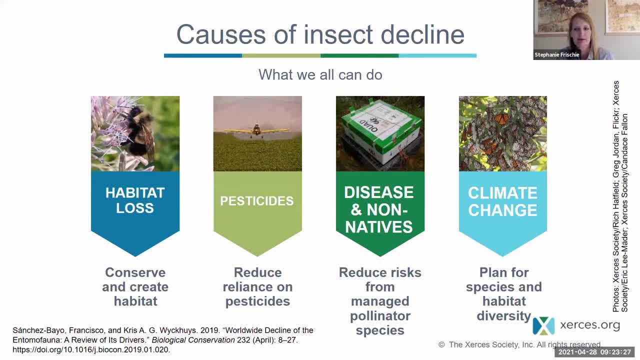 Quality habitat doesn't only support pollinators, it's also important for natural enemies of crop pests, And adding habitat to a farm or an area or a yard will, as well as crop rotation, having a diversity of cash crops and other conservation practices. 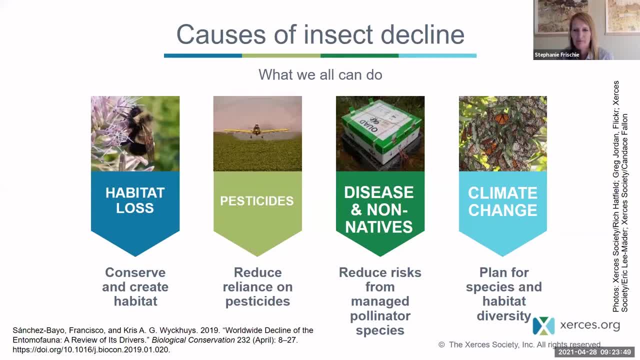 creates a more diverse landscape and habitat. Another major threat: pesticides, and this includes insecticides, herbicides, fungicides, miticides- all the sides. Of course, these can impact invertebrates directly and indirectly, again by leading to habitat degradation or loss. 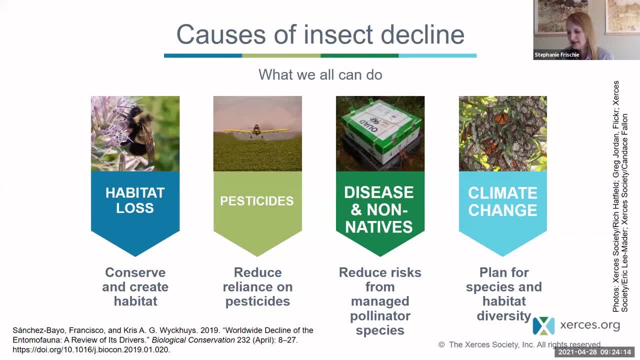 They can also cause non-lethal effects. Many herbicides that have been studied in honeybees have shown- Excuse me, herbicides and other pesticides that have been studied in honeybees have shown how they actually affect the digestive system and the microbes that live in the honeybees guts and 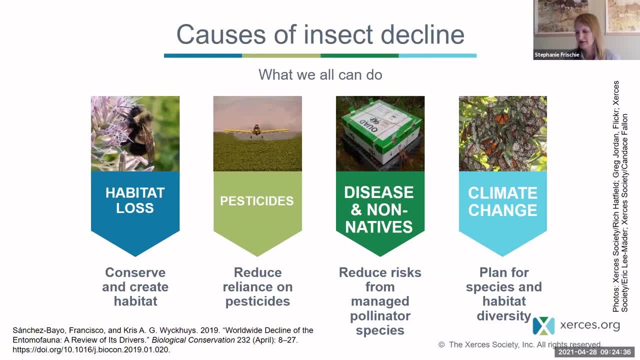 leads to poor honeybee health and overall wellness. So one of the solutions, of course, to that is reducing our reliance and use of pesticides through integrated pest management and also through adding more habitat and more diversity, which which, and that diversification, really deconcentrates the type of plants that pests. 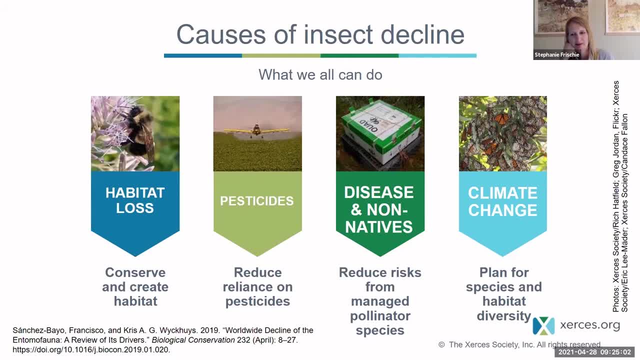 can eat. It also helps to attract and support larger populations of beneficial insects. that again balance any boom and bust pest cycles. Third threat is disease and non-nature. So we have a lot of species that are not native species or managed pollinator species, such 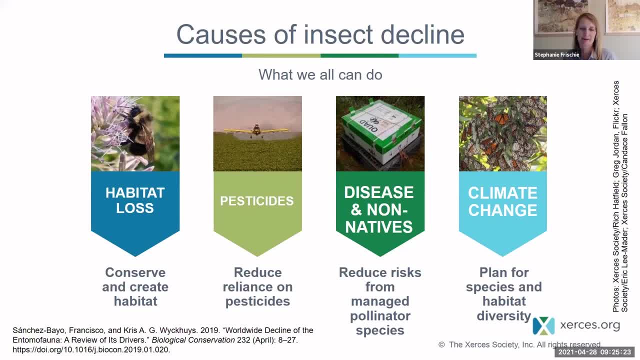 as honeybees or some bumblebee species are also managed as hives and moved around to pollinate crops or to pollinate tomatoes, for example, inside of greenhouses. So these managed pollinators can actually concentrate and transmit disease to populations. 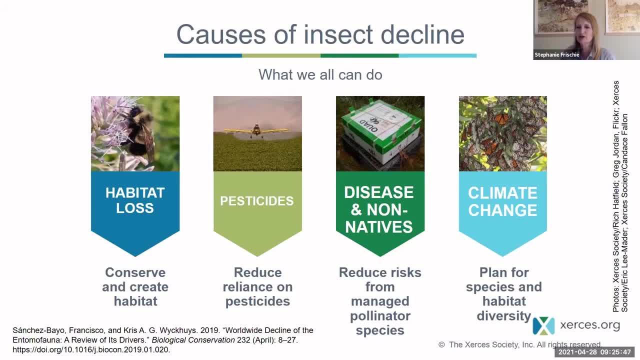 of wild pollinators. So again, trying to create diversity and a place where wild native pollinators can live naturally and pollinate crops is important. And then finally, with climate change, one way to address just all the variabilities and the changing trends and the higher extremes and lower extremes is, again, by creating more. 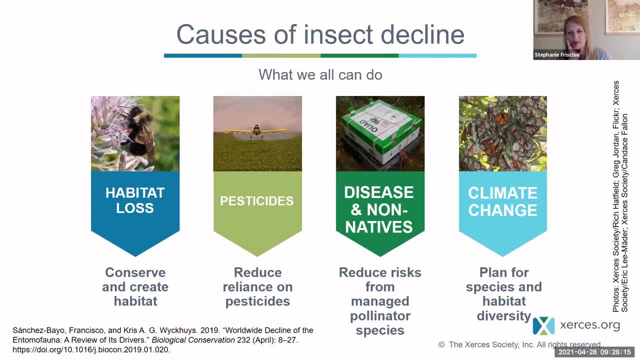 diversity that's better able to withstand drought. So, once again, we have to be mindful of how we use our land in the right way, whether it's the right way to use it. whether it's the right way to use it, whether it's the right. way to use it, whether it's in a place where it's suitable for the climate, whether it's in a place where it's suitable for the climate. whether it's in a place where it's suitable for the climate, whether it's in the right place to consume rainfall, or late or early. 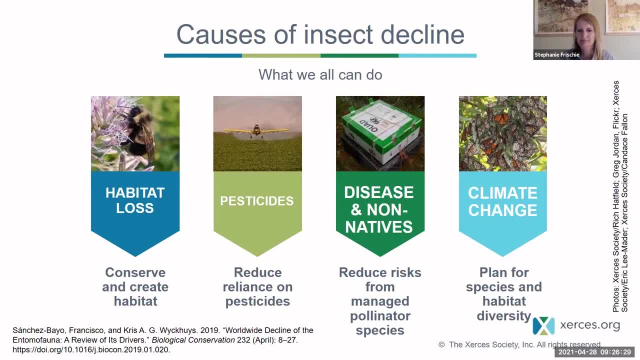 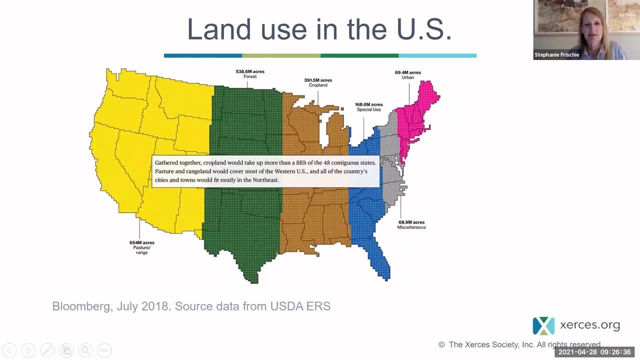 frosts And then also perennial cover of vegetation can help capture and hold carbon in the soil rather than releasing it to the atmosphere. This is a map that we can look at to see how we kind of currently use land in the continental US. It's based on USDA data. 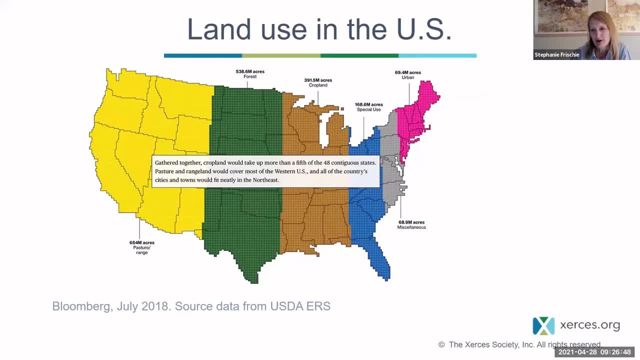 And for the lower 48 percent. So we have a lot of soil Right states. These are grouped by broad use categories and then these colors are overlaid to kind of show relative size. So the yellow represents land that's managed as pasture or rangeland. Green are 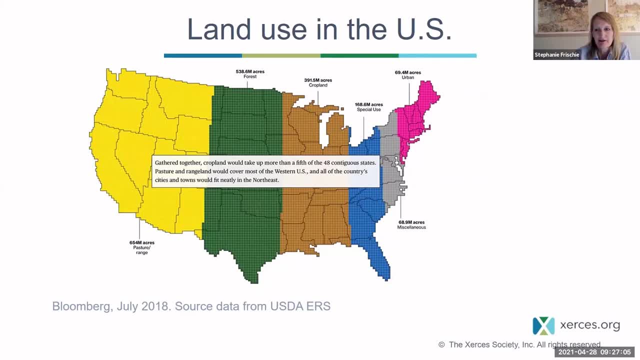 forests or tree farms that are managed for timber and other products. The brown is cropland, Blue is special use. These are kind of actually what was categorized in. here are natural or wild areas, So national and state and local parks, Gray, excuse me, also Department of Defense land and golf. 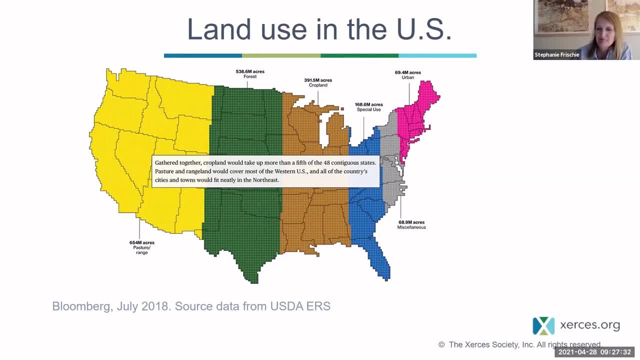 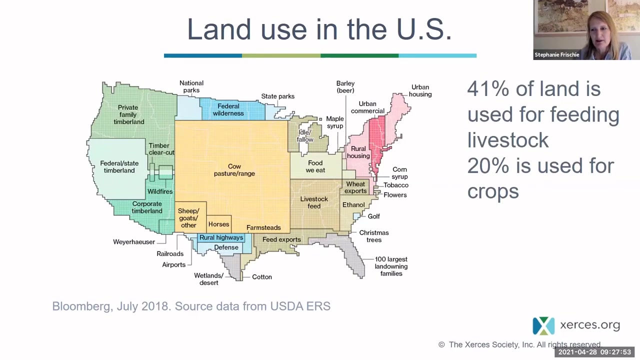 courses And gray was miscellaneous, And then pink is urban areas that are covered in buildings or pavement. And then this is that same data and kind of the same broad color categories, but broken down into some subcategories. And so I think, if we look again here at the yellow, which again was rangeland or pasture for 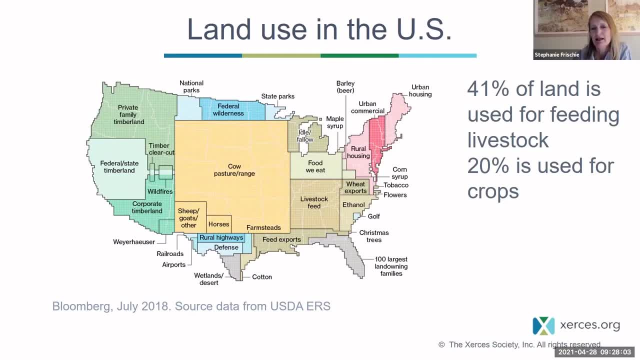 livestock. that was the largest single category, And then all the brown or tan areas are the crops. So all that land that we use for food production is not an insignificant amount. So the message here is just to encourage you. whether you're managing land in pastured areas, in cropped areas or in the pink in urban areas or your yards, each of us can. 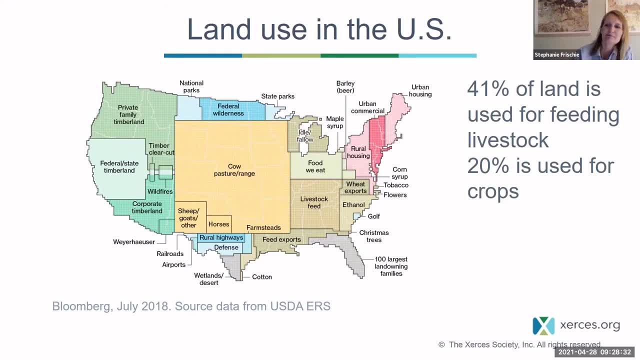 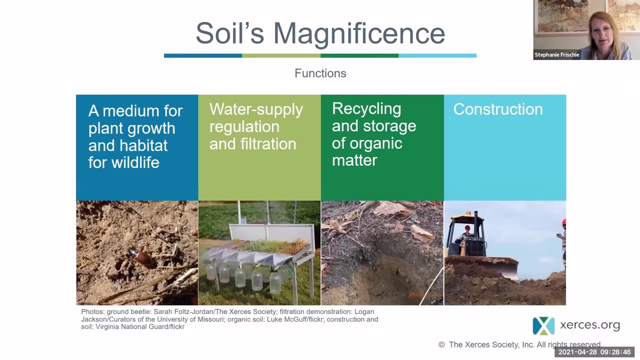 have an impact on how we manage that land: for pollinators, for soil invertebrates and all of that diversity. Okay, next we'll switch here just to a bit of soil basics, And I really want to. I'm calling this soil's. 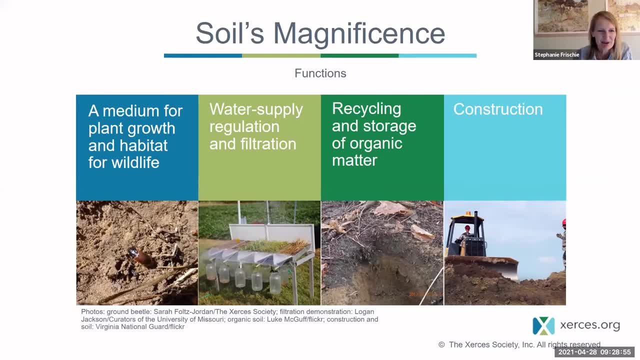 magnificence The more I learn and think about soil. it really is magnificent, Again, from a perspective of human utility. there are several main functions that we can categorize soil as having. It's a medium for plant growth and habitat for wildlife. Soil is also critical to regulate water supply and filter water. Soil is where all the recycling and 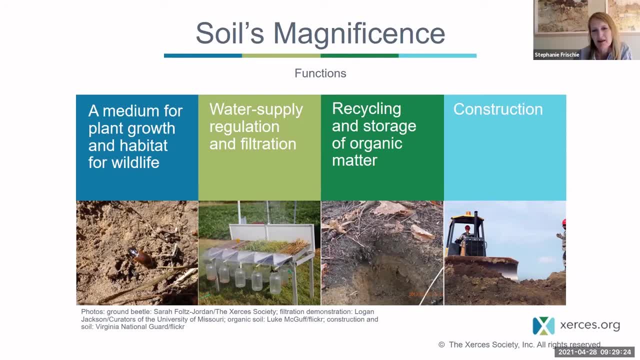 storage of organic matter happens, And then also kind of anywhere we are on land, whether we're directly walking on on soil or in buildings or on roads. soil underlies all of that, And so it's also important for where and how we build or construct things as humans. 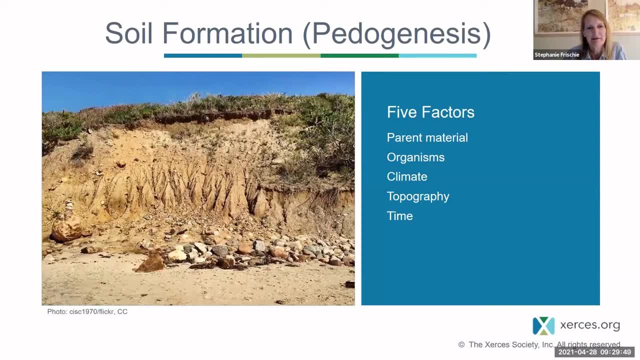 There are five main factors involved in soil formation, which is also called pedogenesis, And those five factors are: the parent material, That's basically the type of bedrock or mineral source that soil is derived from. There are the organisms that live in and among the soil. 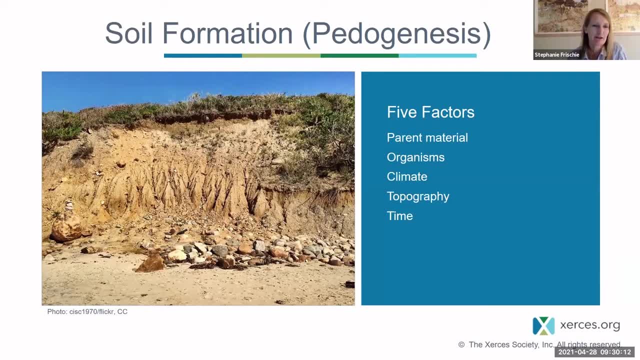 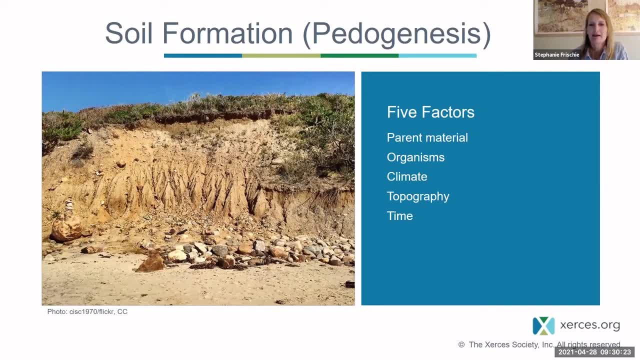 And also help to shape it. This includes plants as well as animals, as well as bacteria and fungi, affects how soil forms, topography as well, And then, finally, time, So the duration or the length of period that all these factors are interacting with each other. 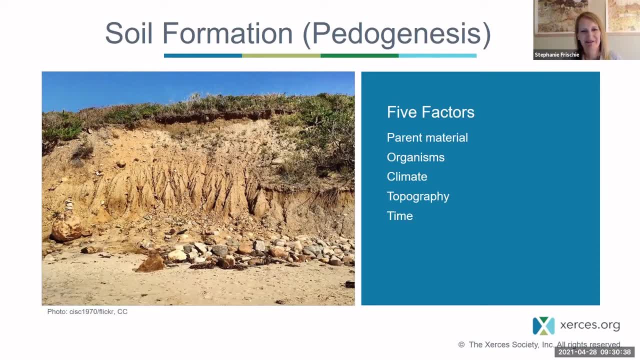 And the photo here, I think, shows the effect of a lot of those factors together. So I believe here- I believe this is on Long Island, So there'd be some granite and limestone as parent material. The organisms here are just plants, but of course there are other animals present. 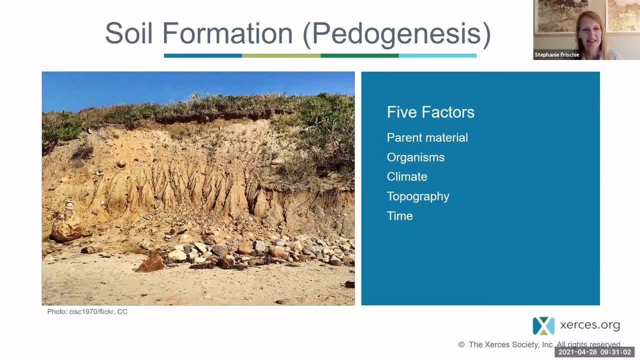 that we can't see. And then topography: you can see here how the larger rocks and pieces are falling down with gravity and then smaller pieces sort out that way. So topography really has an effect in terms of how gravity acts on these particles. 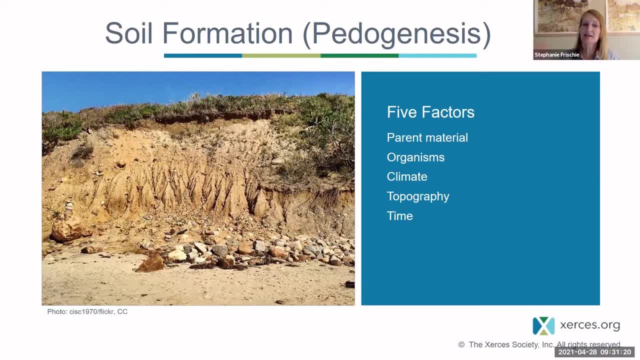 You can also see how processes are working to form soil and processes that are considered things like weathering or organic matter accumulation or actually loss of organic matter as well. So that's just a bit of a refresher about the interactions of these different factors. 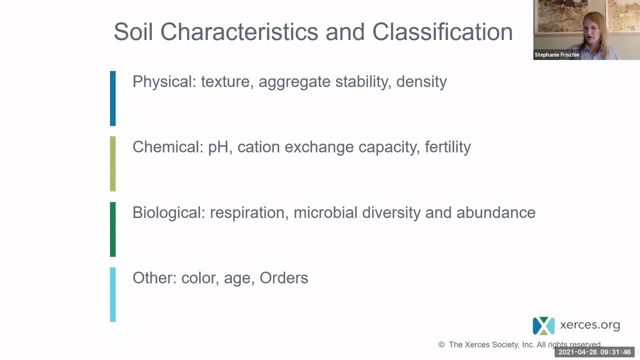 and how soils form. There are also several ways to describe and categorize soils. Physical types are talking about texture, aggregate stability, bulk density of soil. Some chemical characteristics are the pH, the cation exchange capacity and other measures of fertility. 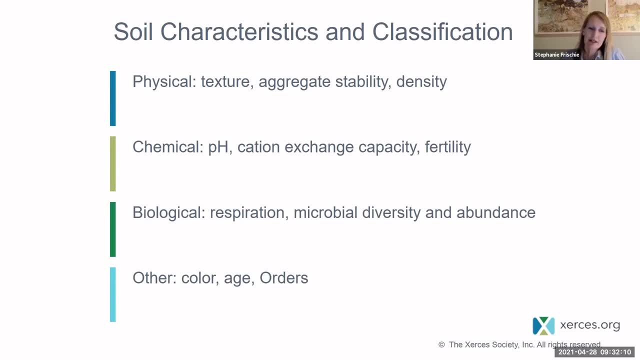 There are biological ways to measure categorized soil, such as through respiration or measuring material, measuring microbial diversity and abundance, and then other ways that soils are categorized, maybe through their color or the age of soils. and there's also a whole soil taxonomy where soils are organized into orders and then also into series. 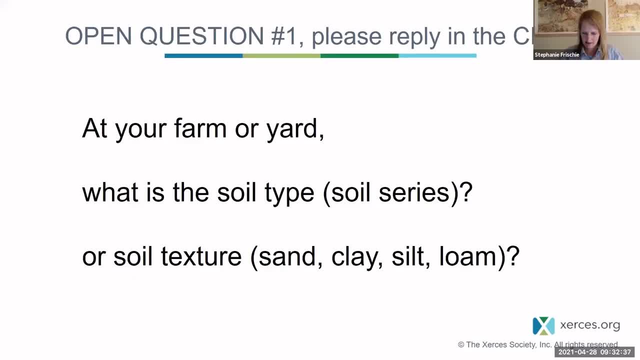 and here we're going to just take a little pause and have Liz open the the chat and we've got a question for you. it's got an open-ended answer and we'd like to ask you to please reply in the chat. so, at your farm or yard, what is the soil type? and there I'm we're mostly interested in if 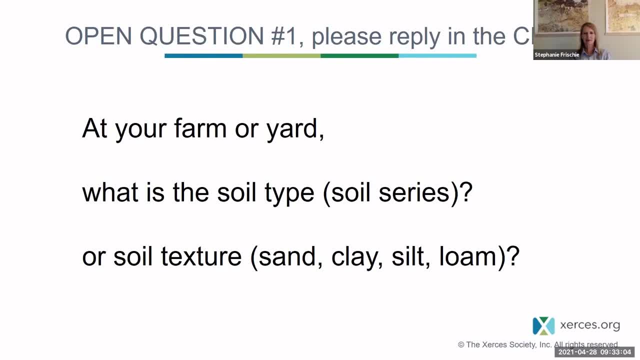 if you know what soil series your farm or yard is. additionally or alternatively, we'd also like to know what's the soil texture like at your farm or yard, and so that would be whether it's more sandy or there's more clay, maybe it's a little bit rocky or there's a lot of silt, or 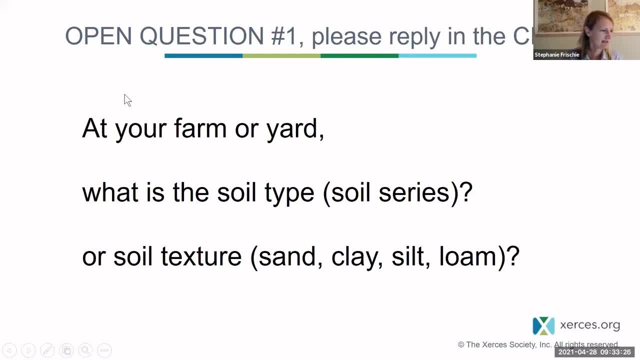 loam texture. so go ahead and we'll take a little time to to let people fill that in in the chat. um, all right, we've got all kinds of good responses coming in here. I'm not going to go through everyone but, um, we're seeing Siltilone, Claremont, Cincinnati, Iowa, So those names are different soil series They're. 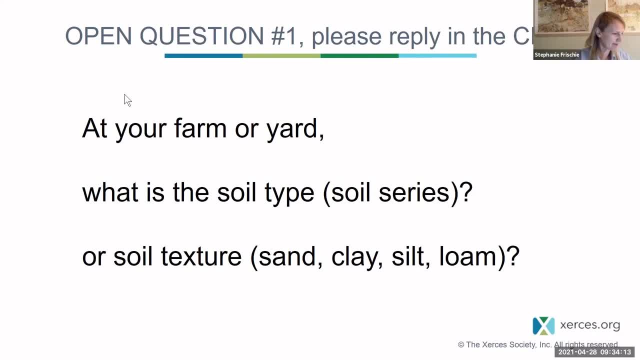 often named after the location where they were first described by soil scientists, And then you can search online and actually find descriptions of soil series Mollisol, that's one of the soil orders, So in soil taxonomy words that end in that suffix S-O-L, which is related to our word for soil. that's how you can identify. 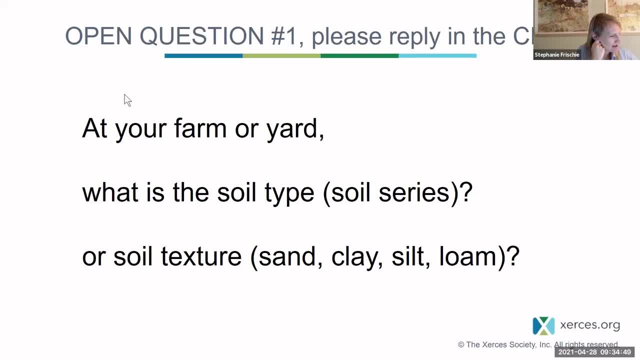 when someone's talking about a soil order. So molluscs are typically soils that formed under grassland vegetation and they actually make for rich, fertile farmland. So a lot of the soils in the Midwest and sprinkled throughout other areas that were historically grasslands. 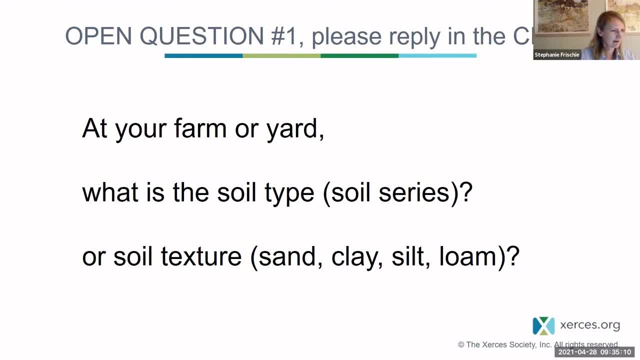 have these molluscs. Okay, thank you everyone for sharing about the soils where you live in the chat We're gonna, I think, Liz, you can leave that open or close whatever makes sense there and we'll move on here again. 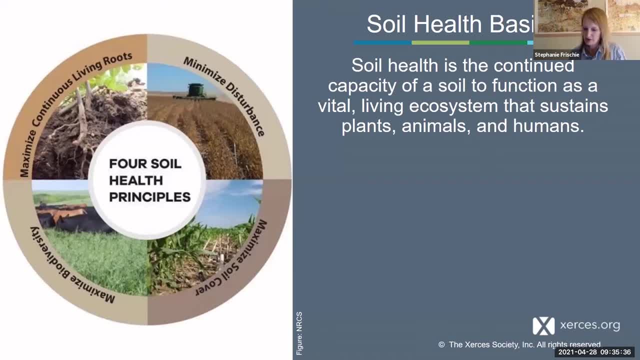 And now talk a little bit about soil health. So, beyond simple intuition, one technical definition of soil health is the degree to which soil is optimized to support various ecosystem services. There's also the definition by John Doerr and Michael Zeiss written here: it's the capacity. 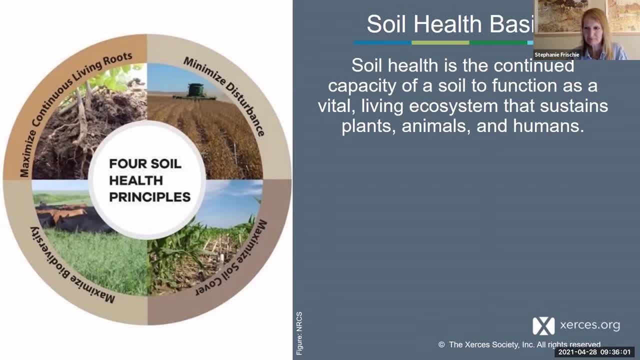 of soil to function as a vital living system within these different land use boundaries, to sustain plants and plants for the environment, the basis that they are used to. So the application in animals and humans. One regenerative farmer that Xerces has worked with: 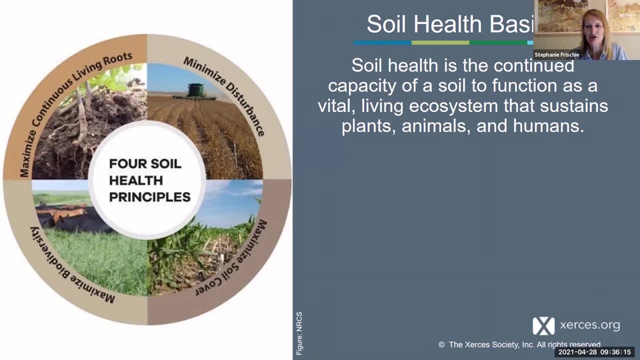 has described it as when he's able to decrease external inputs while maintaining good and stable crop yields. I'm gonna have to jump a little bit ahead here for time, but we've got the four soil health principles featured here on the right. Two of them are really focused on protecting soil. 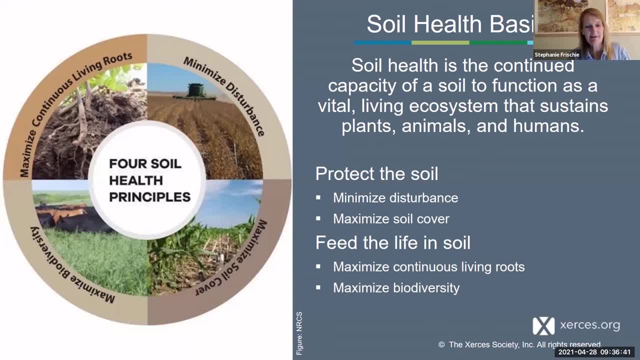 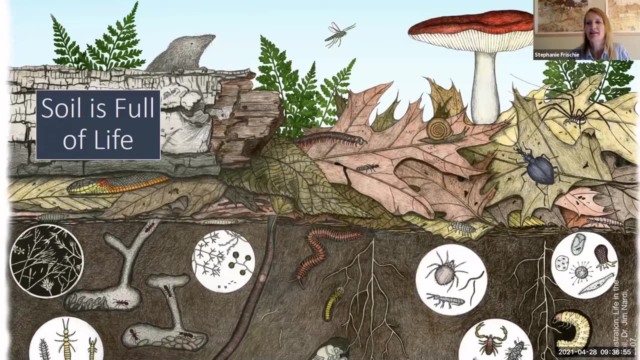 and on the left two are focused on feeding the life in soil, And we'll talk about these again later in the session, but I wanted to introduce those here and then get on to soil invertebrates. So this is really the focus for our short course. 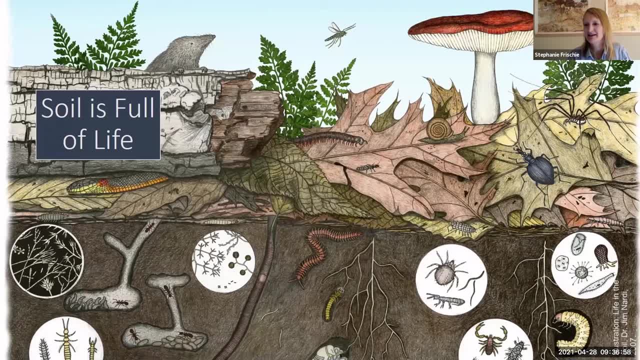 that soil is full of life, from the tiniest microbes- bacteria, fungi and protists- and increasing in size to mesoinvertebrates, macroinvertebrates and also, of course, including land plants and vertebrate animals. This slide is just a preview, as we're being ready. 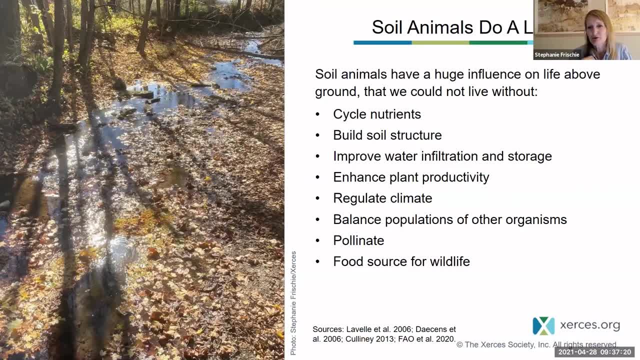 to go into the profile section here in module three. So just wanted to highlight all the roles that soil animals, especially soil invertebrates, play. We could not live without all these functions and roles. And again, one teaspoon of soil has been estimated. 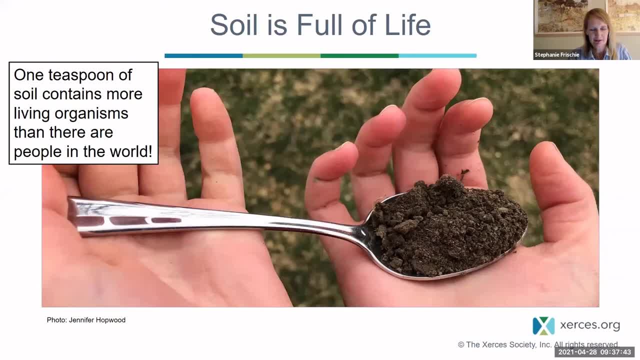 to contain more living organisms than there are people in the world. This is really talking about the estimate of 1 billion bacteria, several thousand protozoans, So these very tiny, microscopic animals, and then getting into nematodes and many other fungal filaments and other tiny animals. 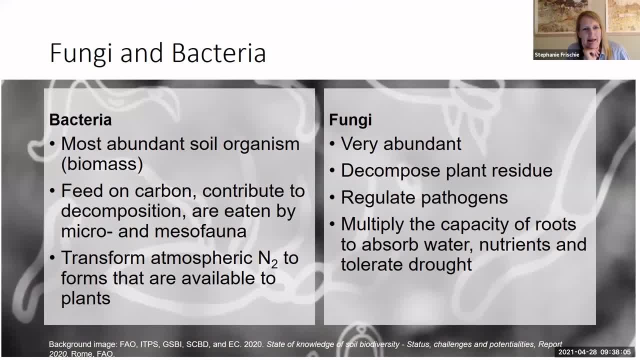 Just quickly. we're not gonna talk much more about soil, much at all about bacteria and fungi, but they are an important part of soil life. Bacteria are the most abundant soil organism. They feed on carbon, contribute to decomposition and they are eaten by the micro and meso fauna. 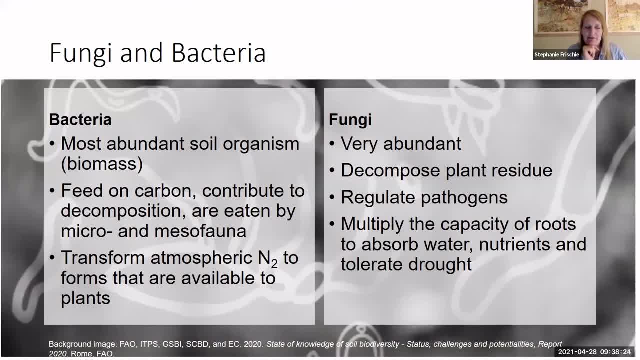 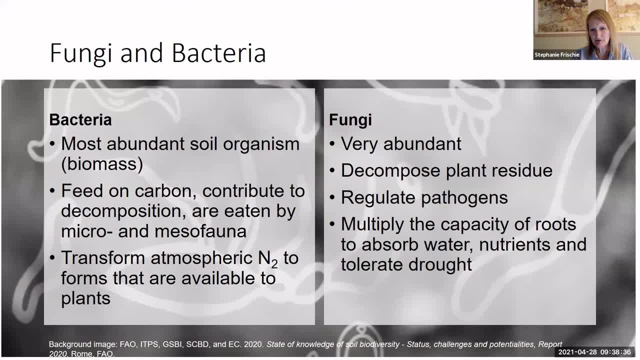 decompose the plant residues. decompose the plant residues and break it down and make it available for other groups. They help regulate pathogens and they also multiply the capacity of roots to absorb water, nutrients and tolerate drought. And the reason why I wanna show this image. 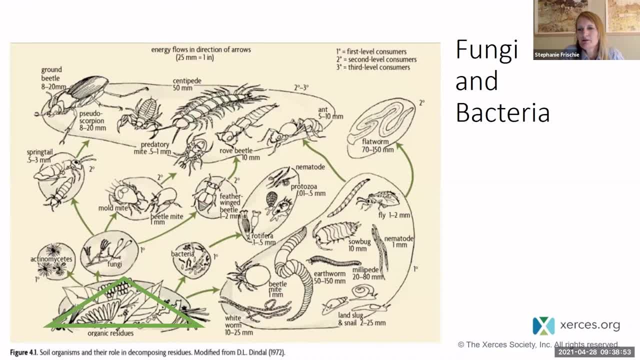 is to illustrate the flow of energy in soil ecology. So the green arrows show the direction and relationship of energy flow between these groups of organisms. This does not show living plants and their roots or larger animals, but it really zeroes in on the organic residues. 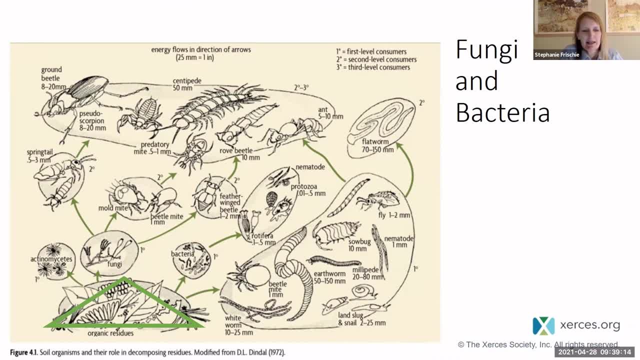 mostly dead or shed material from plants and dead animals as well. That's the green triangle at the bottom left And then if we look at bacteria circled in orange, we see this movement or transfer of energy and decomposition. but these are short networks. 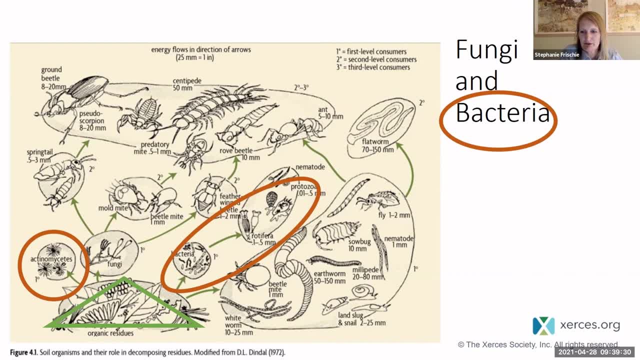 They don't really connect directly to the other groups that are pictured here. And then, if we look at fungi, they're very active. And then, if we look at fungi, they're very active. And then, if we look at fungi, they're very active.